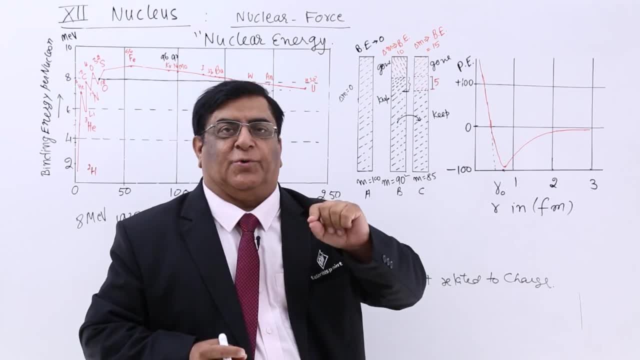 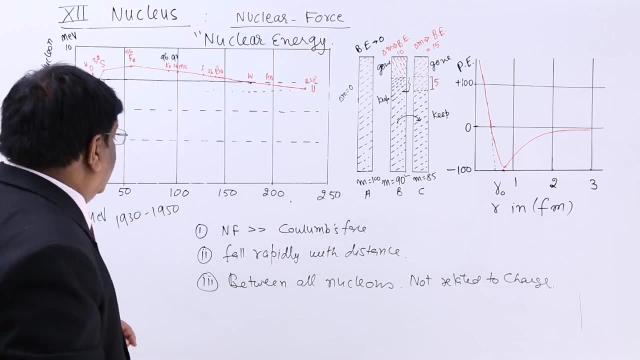 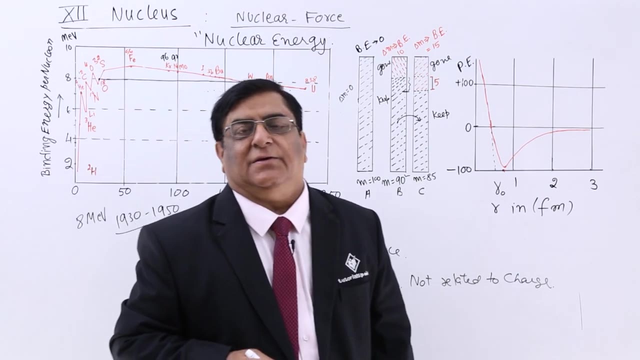 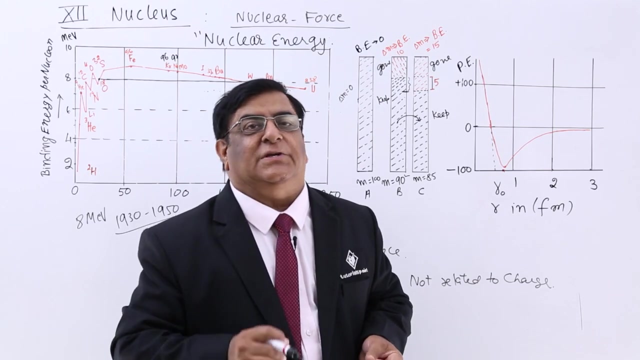 and R. This graph was made for potential energy by various experiments which were done in atomic field During the year 1930 to 1950, many experiments were done and some you have seen that Rutherford experiment and after that, After that, many experiments were done to find out the nuclear energy between nucleons and it is found that it changes with the occurs between two nucleons center to center, that the distance between the two nucleons is 0.8.. We find that when this distance is nearly 0.8, Fermi. 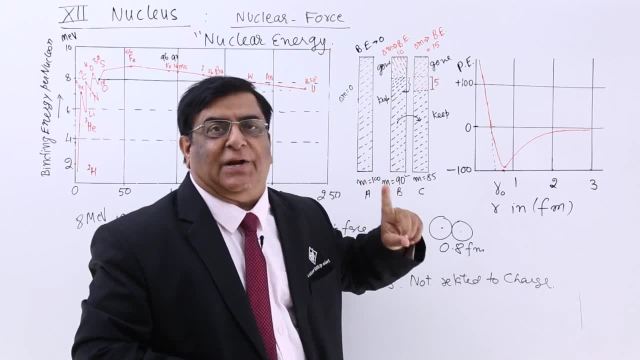 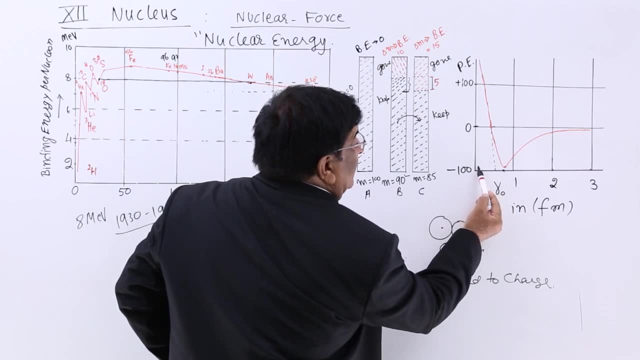 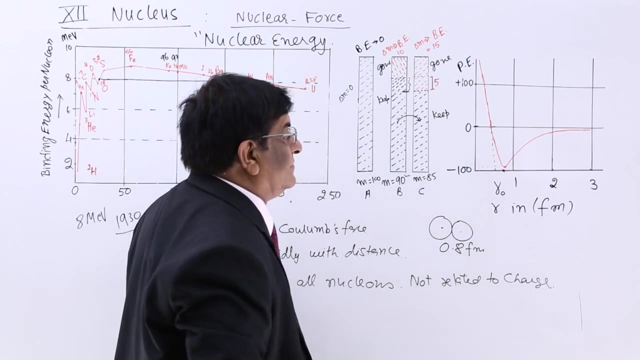 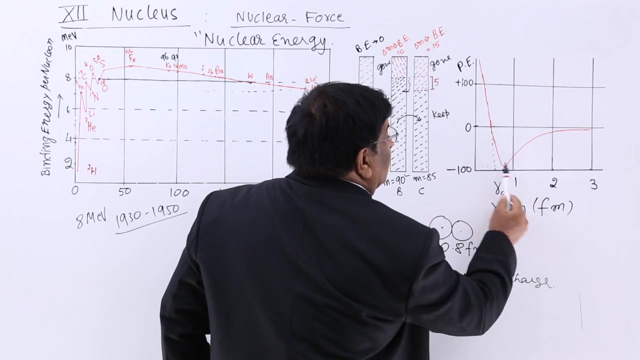 the attraction is maximum and the potential energy is negative. It has this maximum negative value when the distance is r0.. Now what happens when the distance is increased? When the distance is increased, still potential energy is negative, negative, negative, negative. 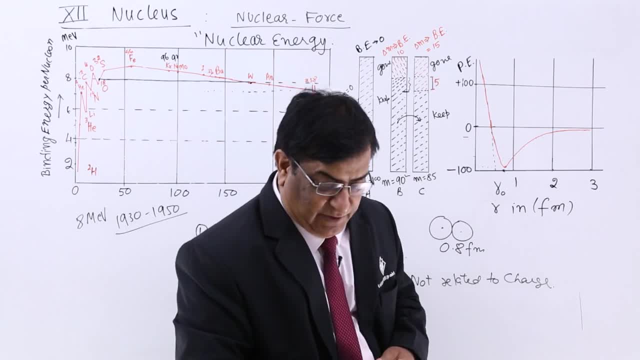 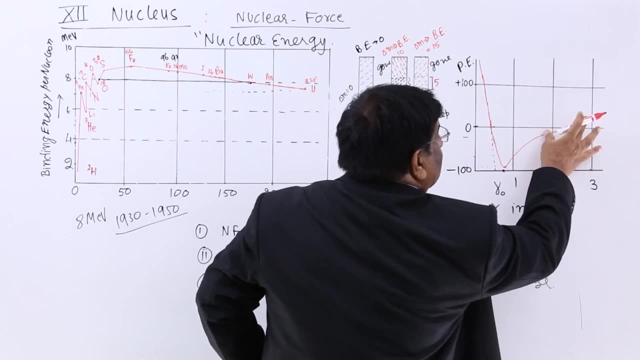 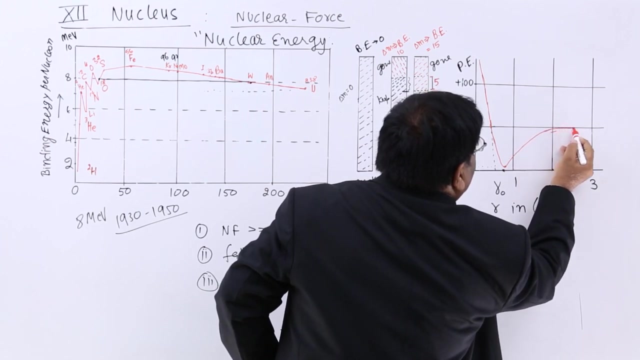 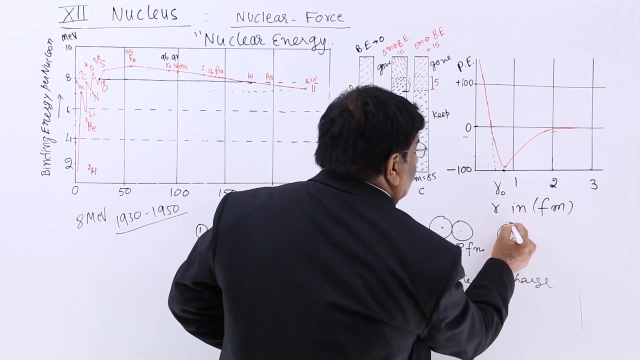 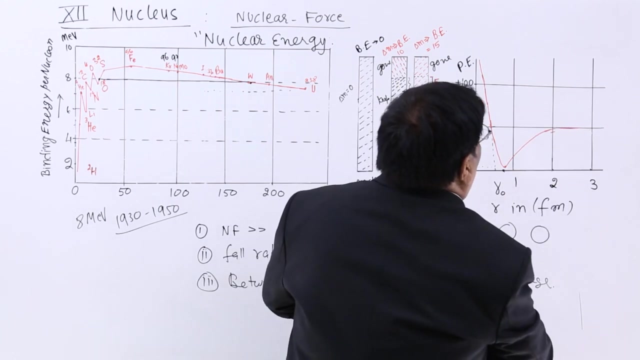 This shows that there is still a force of attraction between them, but the energy decrease a lot. and this, even this, will go like this. That means the moment it cross this distance, more than 2 Fermi, this, this: the force of attraction has become very, very less, or the energy has become very less. 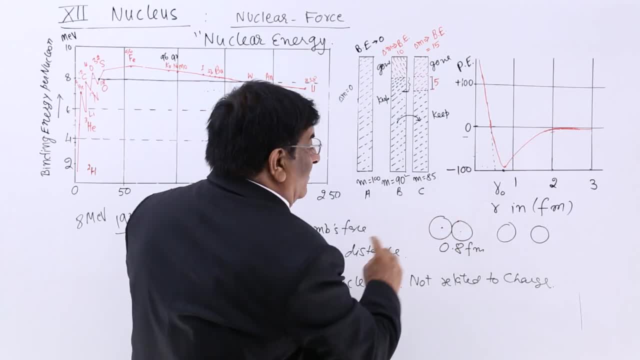 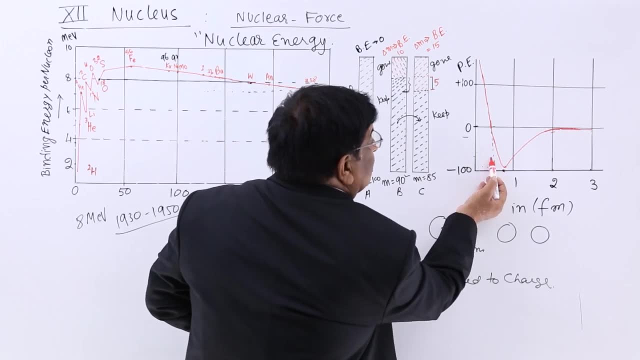 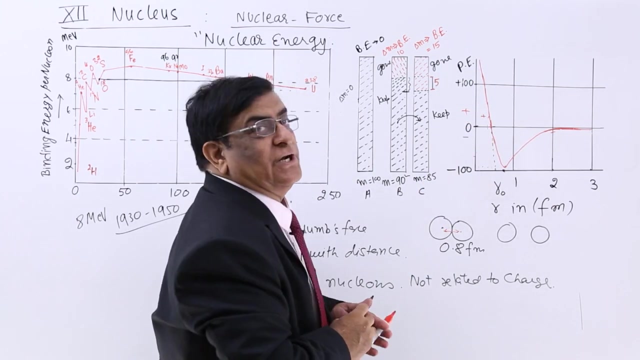 Okay, This happens. Now if we compress them and this distance become less, what will happen? If distance is become less, the energy become positive, and positive energy shows what The force of repulsion. So if the distance become less, the force is repulsion. 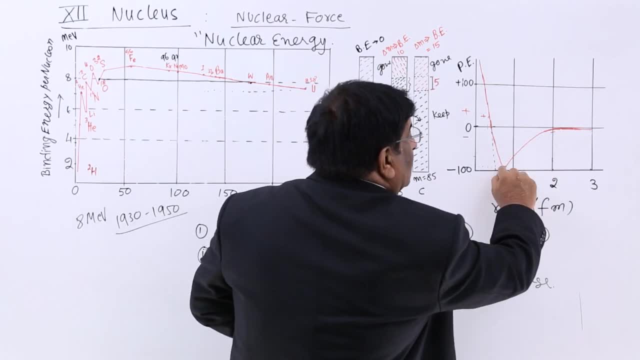 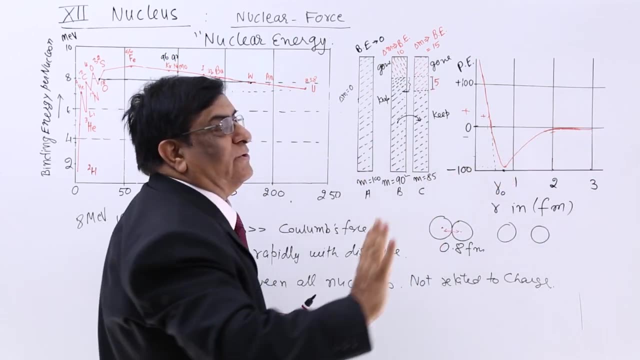 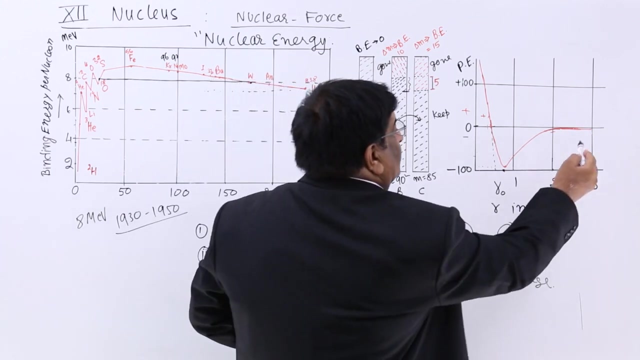 If the distance increase a little up to 2, the force is all attraction. If the distance is more than that, the force become almost 0, there is no force. So we can say nuclear force is a very short range force, only say this much. 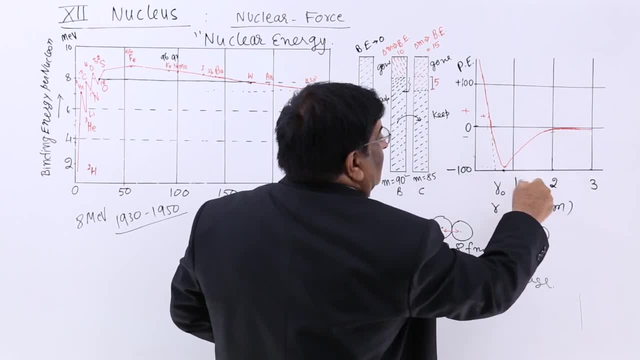 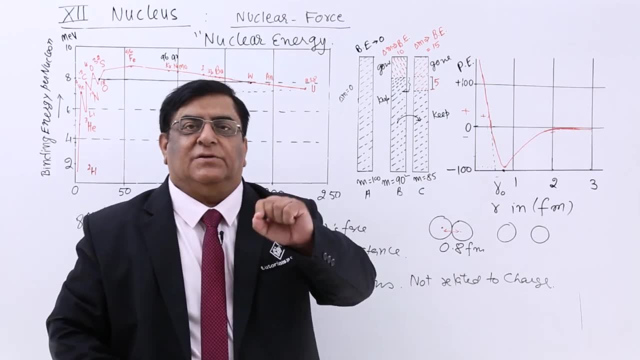 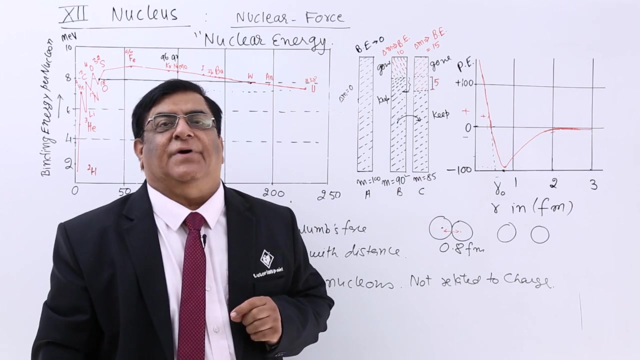 It plays from 0 to 0 within 2 Fermi. that is all. that is why it is known as short range force. Now, this nucleus to nucleus force, The nature of force. Okay, This force is a very strong force compared to Coulomb's force. 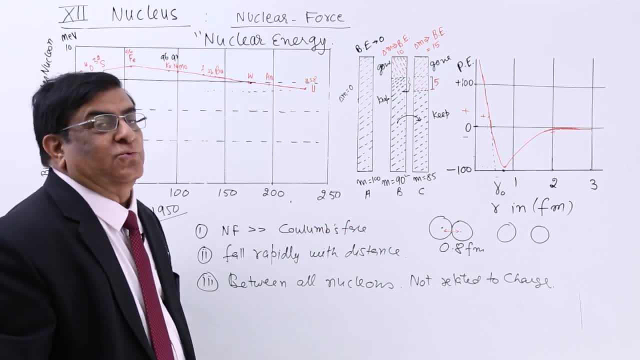 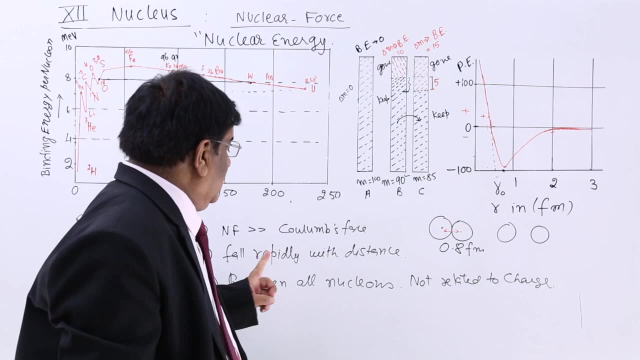 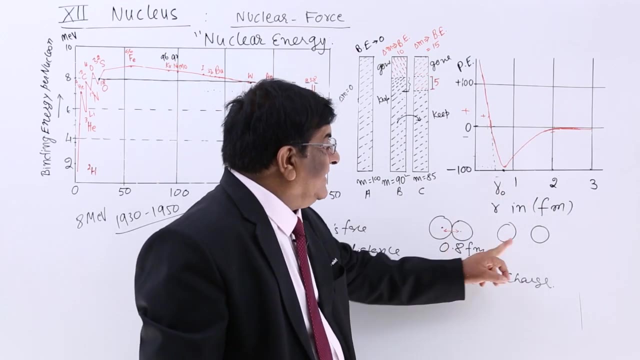 So this nuclear force is very large compared to Coulomb's force. that is 10 times larger than Coulomb's force, But at the same time it is a very short range force. It falls rapidly with the distance. If the distance increase, the force decreases a lot. 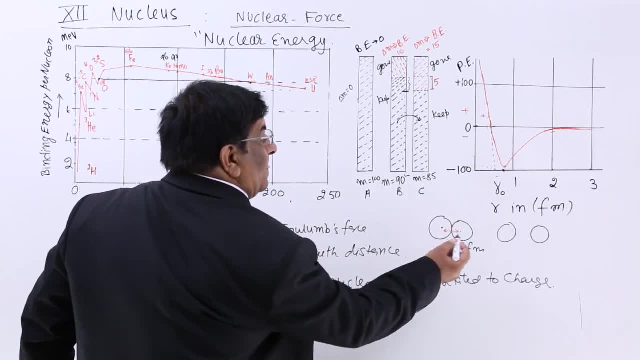 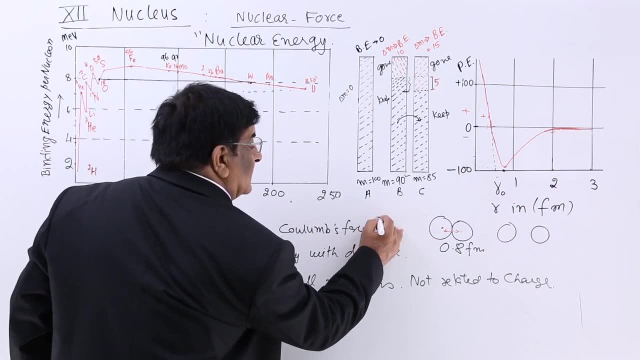 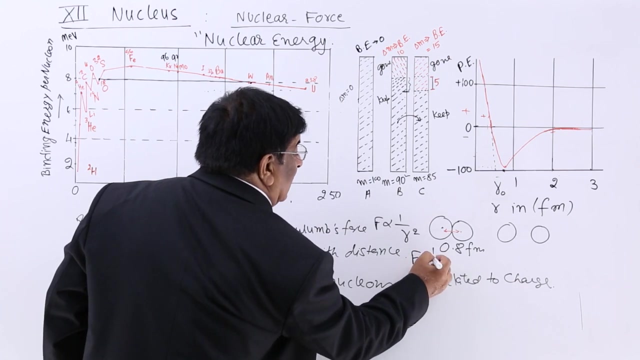 There is a lot of fall And if this distance is more, the force is almost 0. But in Coulomb's we see the force is inversely proportionate to square of the distance. Here it is much, much larger than that. 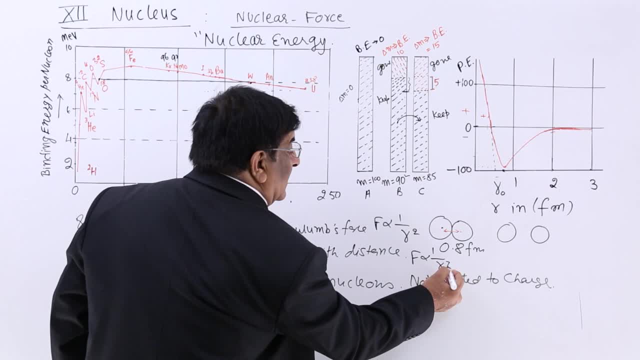 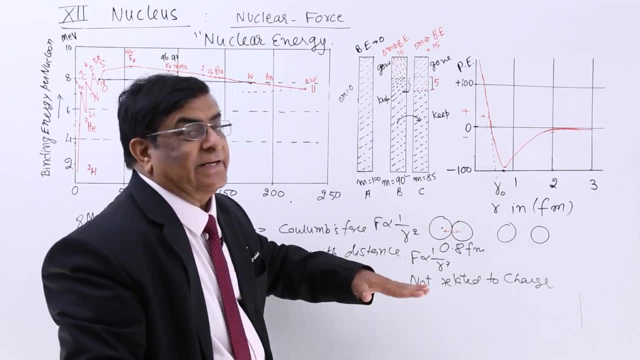 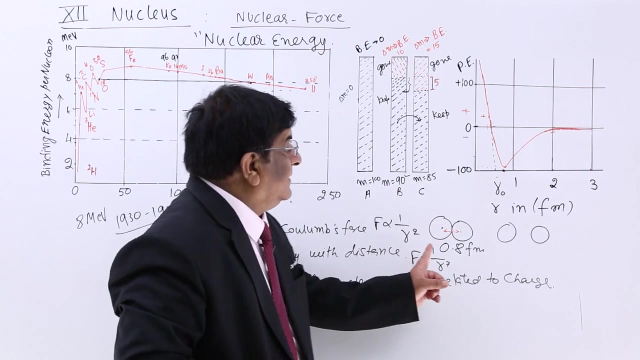 We do not give any commitment how much it is, but it is changing and it is changing very sharply. A small change in R will decrease the force very less. Now this force, is it different for proton to neutron, proton to proton or neutron to 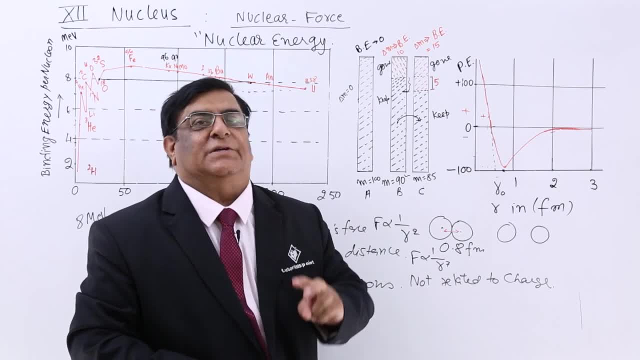 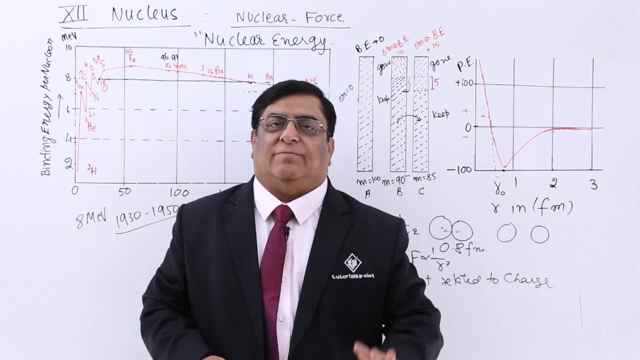 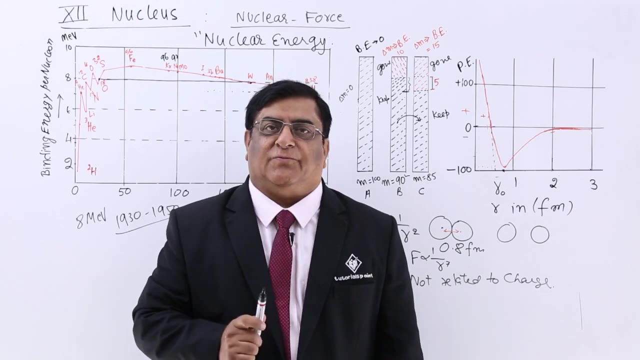 neutron. Answer: no, This force is same whether the two particles are having 0 charge, positive charge or plus, and 0 charge Does not matter. That is why it is a different type of force We have studied so far. Gravitational force is one type of force in which masses are required. 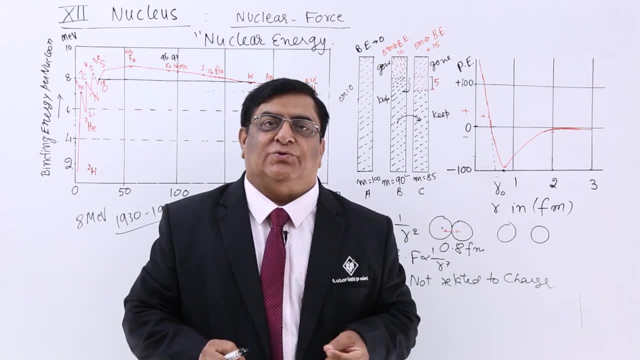 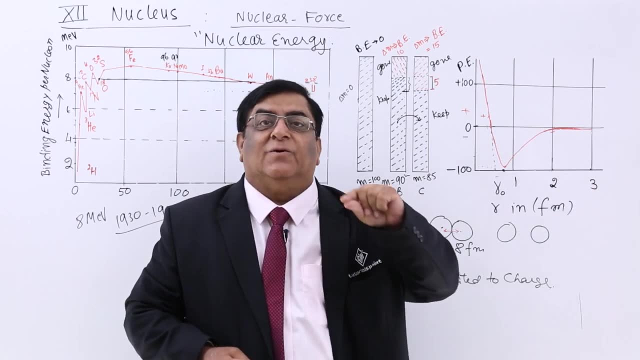 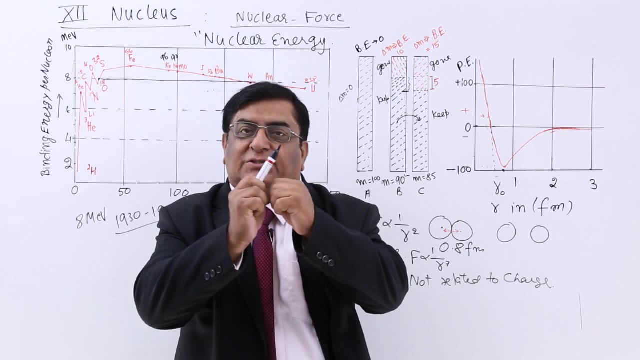 The other one is electric charge force in which charges are required, electrostatic force In nucleus. what happens? It is within the nucleus and one has to be a nucleon. And this force is such a large force that Coulomb's force and gravitational force both. 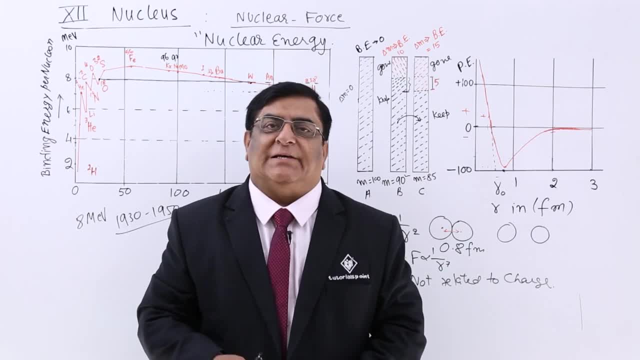 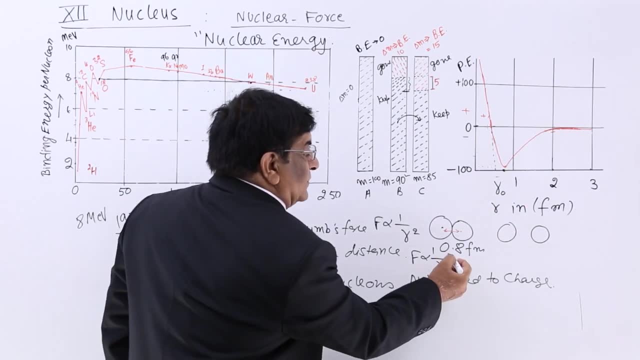 are negligible before then. But only thing is, it is exerted when they are very close to each other. 0.8 Fermi of this much, Then only this is applicable, and it is applicable up to 1 Fermi: 1.5 Fermi. 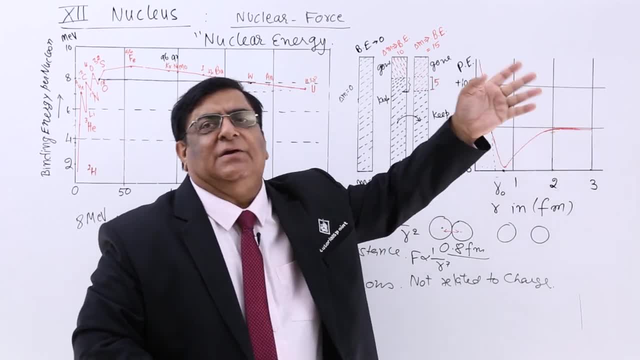 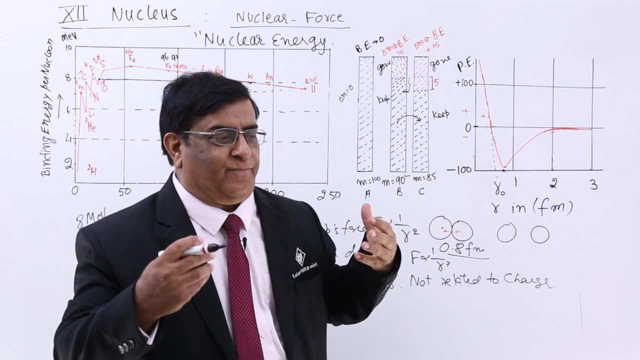 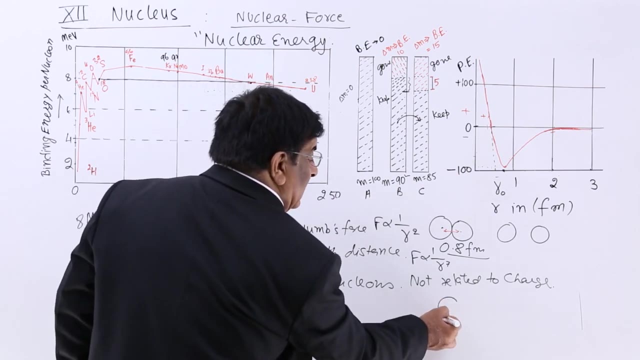 But when it becomes more than 2 Fermi it becomes almost 0. So this is nuclear force. Why This force was significant? This force is significant because it has a very large charge, Because otherwise we cannot explain that why a proton and another proton should be together. 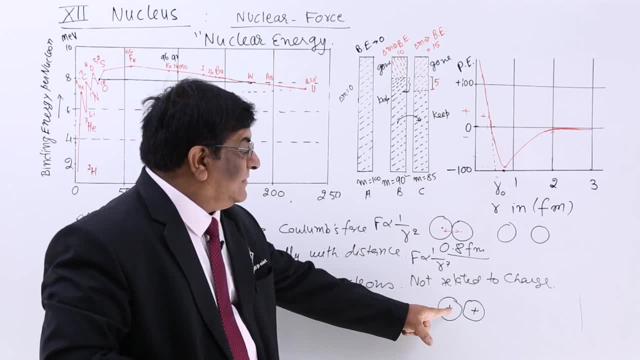 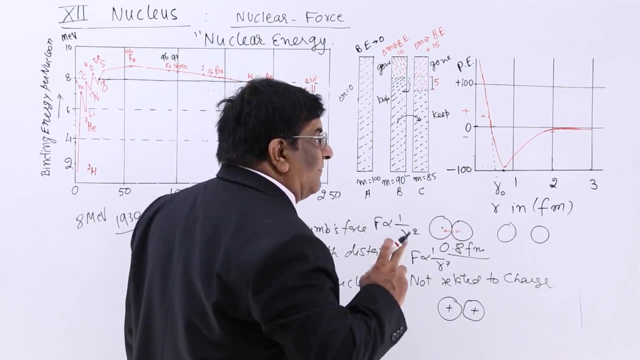 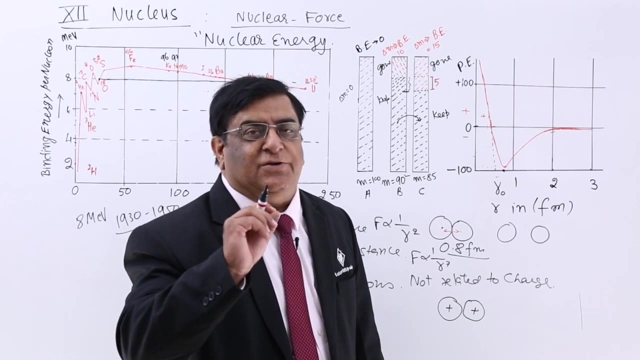 in a nucleus. We know that there is a very strong repulsive force between the two protons. Now we have not seen any nucleus which has got only two protons. The smallest nucleus we see with two protons is helium, which has got two neutrons also. 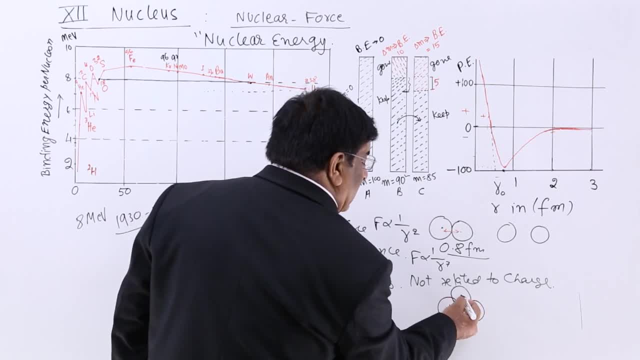 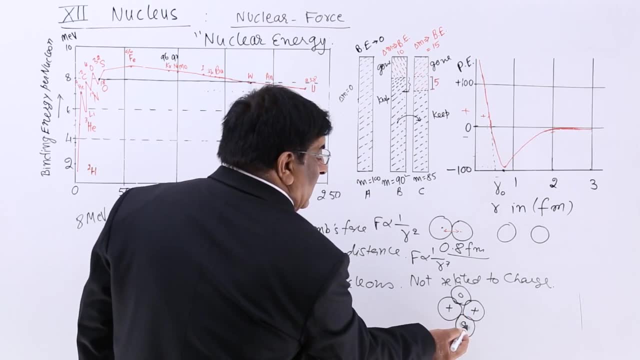 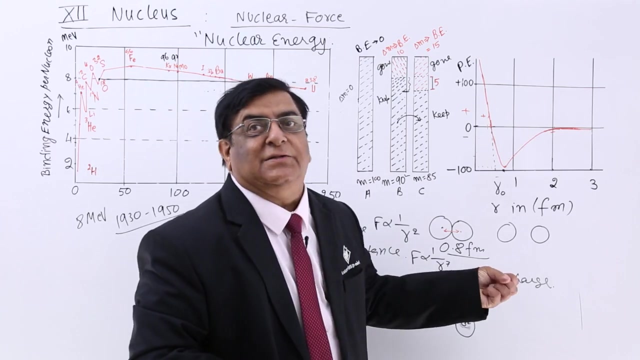 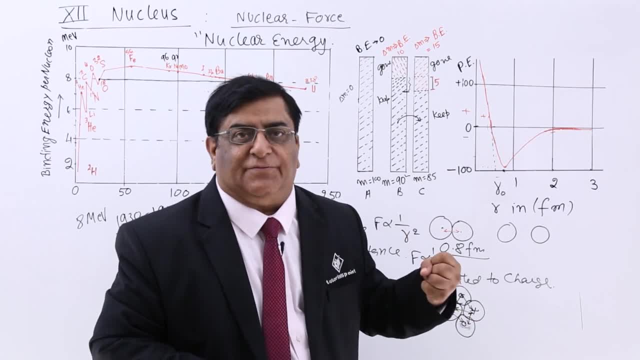 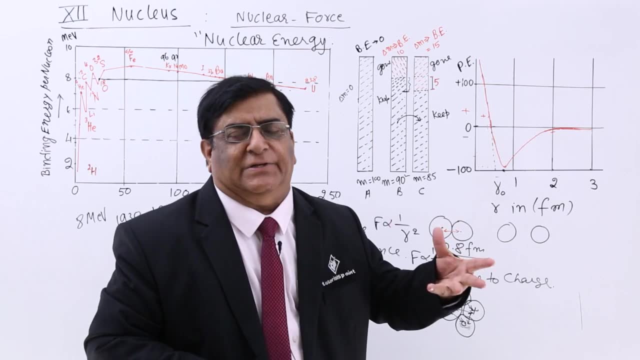 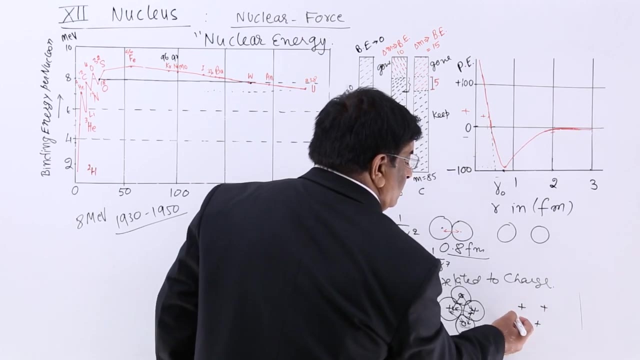 So now you see, there are forces of attraction which are much, much larger than a single force of repulsion. We can go for higher one, like carbon. Carbon has got six protons: 1,, 2,, 3,, 4,, 5,, 6.. 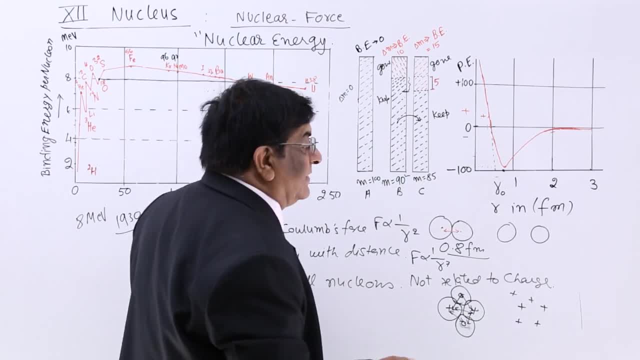 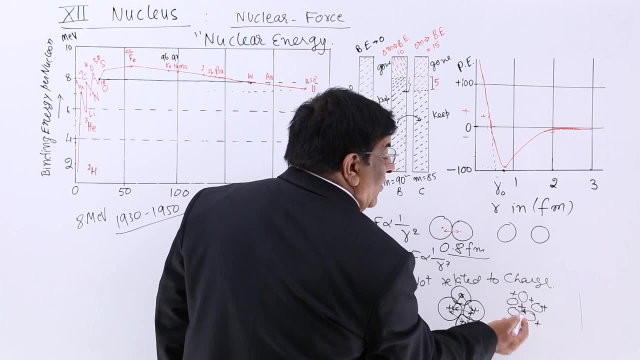 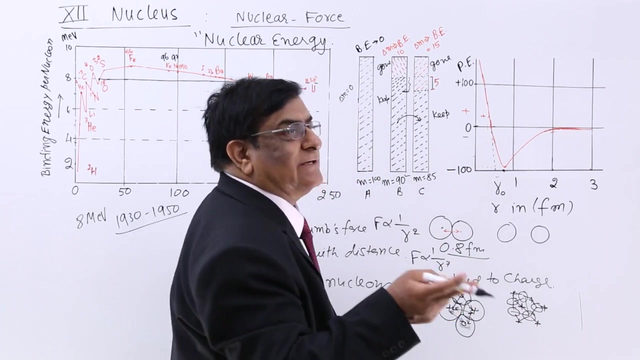 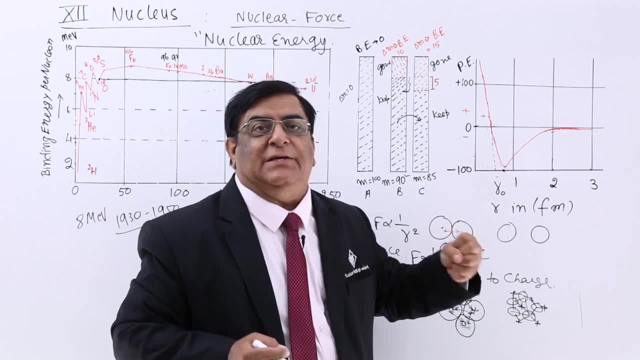 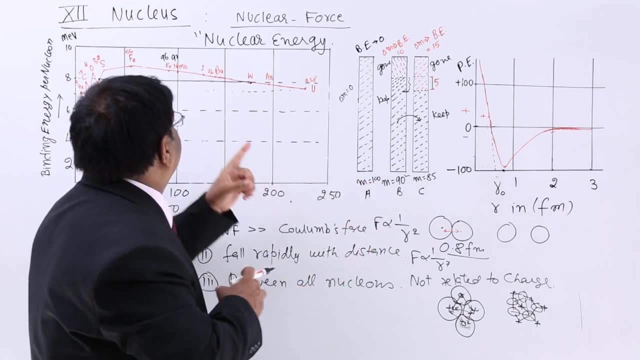 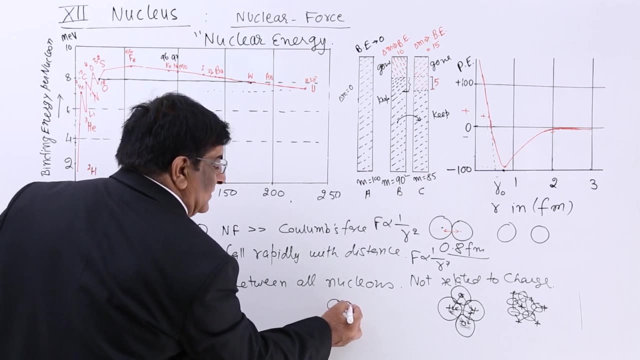 So this is, this gives stability to the nucleus. but another thing: if it grows larger, larger, larger, What happens if it becomes very large, like this? Now, this and this, the distance is, this is plus, this is plus. 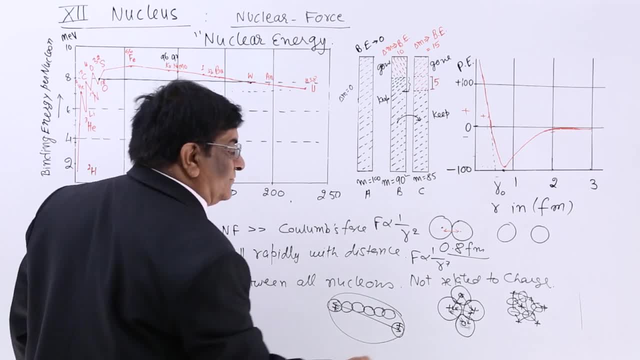 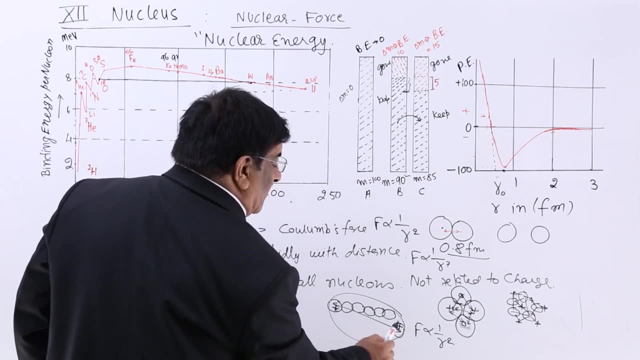 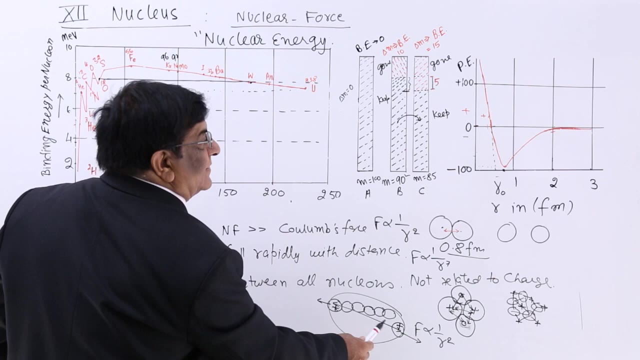 They will have a force of repulsion that f is proportionate to 1 upon r. square r is quite large, So this force of repulsion will be less, But there will be repulsion. Now, what about force of attraction, which is nuclear? 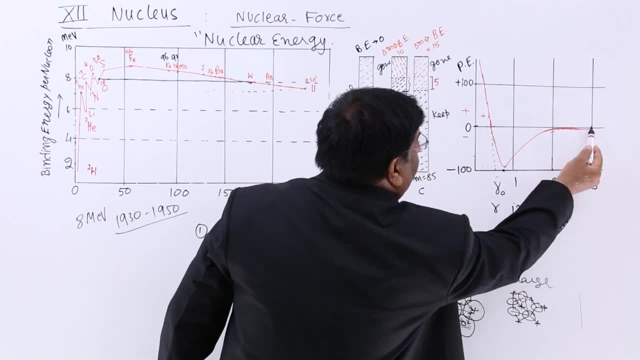 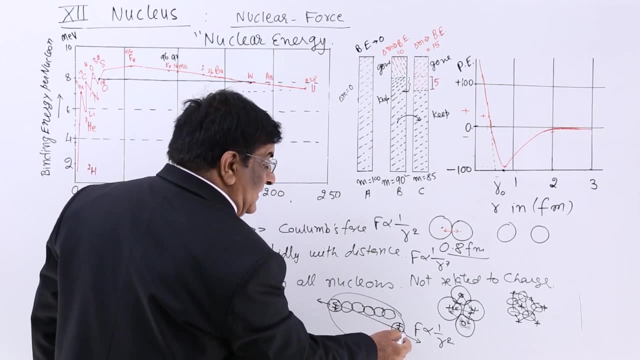 Nuclear force. if the distance is more than 2 Fermi, 3 Fermi, nuclear force is 0, no force, very less force. So when the size increase, then nuclear force become weak, weaker, weaker, weaker, weaker. 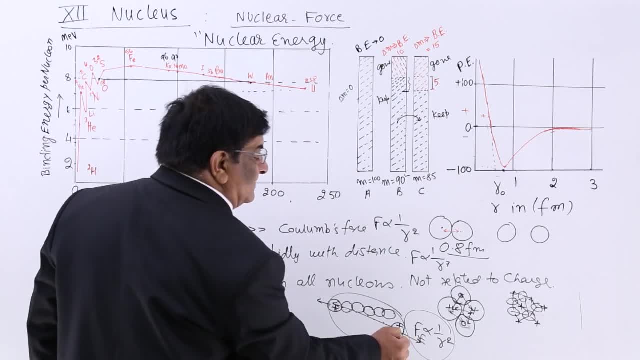 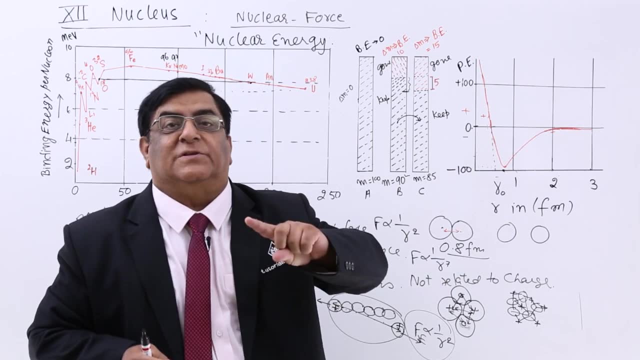 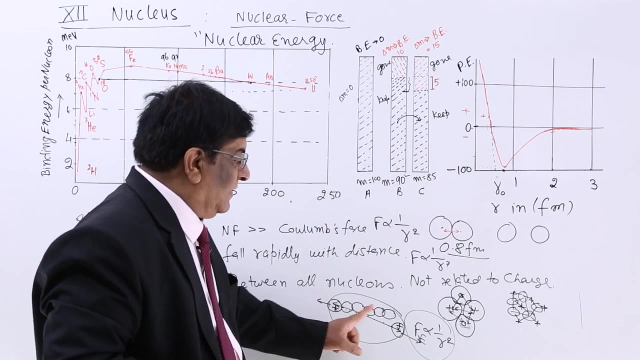 it has become weaker than the electrical force. If it has become weaker than the electrical force- and electrical force is repelling- then who becomes the prominent? Now, repulsion is prominent and this will break. This will break and this will be ejected out. 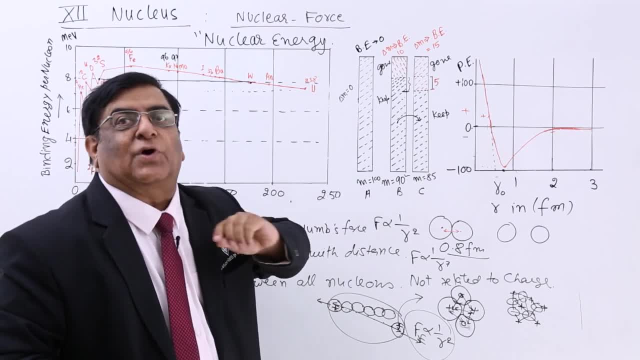 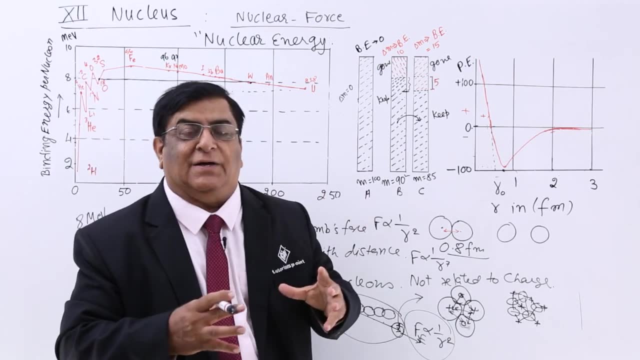 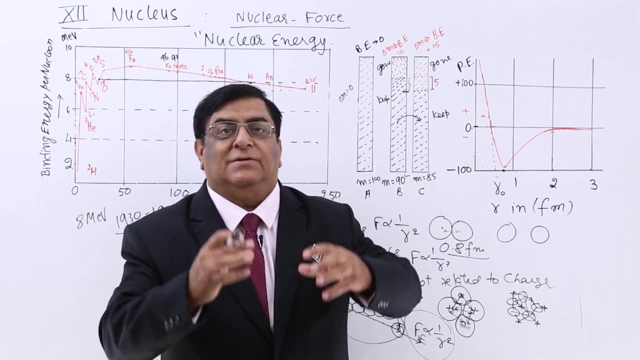 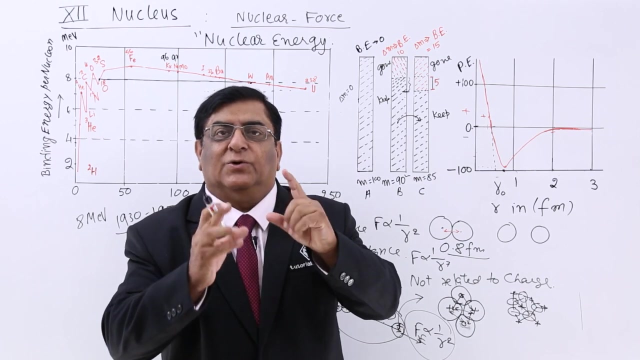 This jump out because it is ejected from the nucleus. This happens, So there is a limitation of this phenomena. That nuclear force bind them together. It do bind them together against the repulsive force of protons, but the size limited. When the size become large, Coulomb force become little weak, but nuclear force become 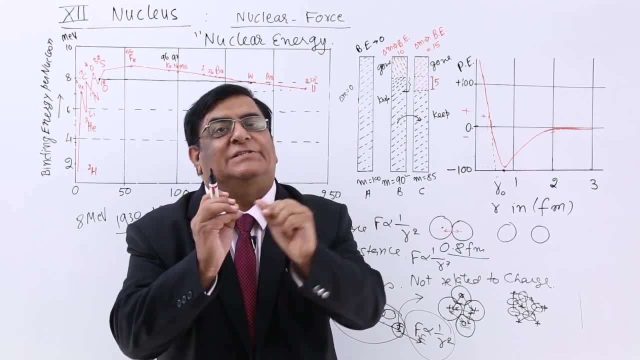 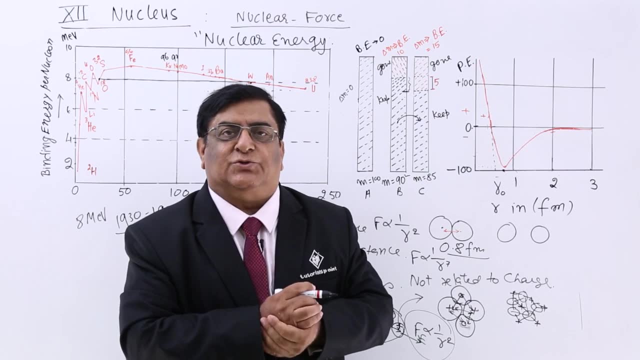 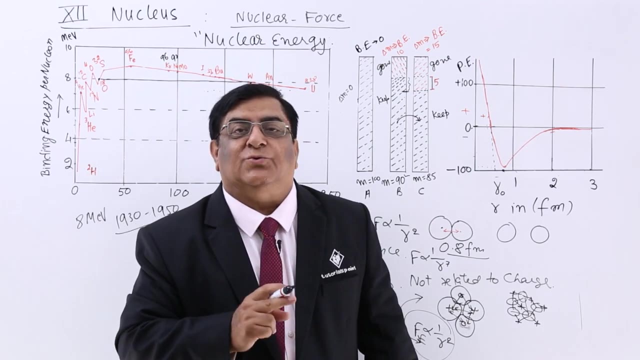 very weak. Therefore Coulomb force eject out the positive. We call that phenomena as radioactivity. We will come to that in the next chapter. So this is the limitation of nuclear force and this is the limitation why we do not get very large nucleus. In our nature the largest nucleus we get is U238, and if the particles are more than 238, then number of protons will increase and they will be so many that repulsion force will be very large, Larger than nuclear force of attraction, and in that case it will eject out the protons. 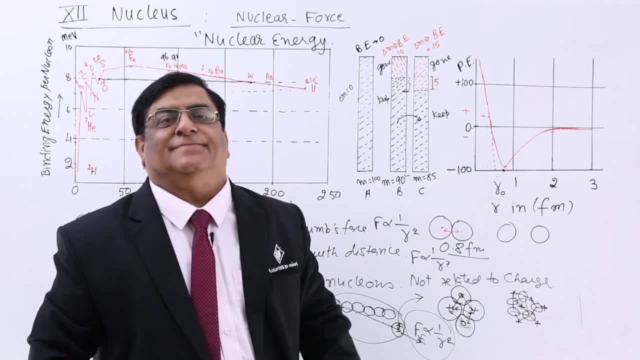 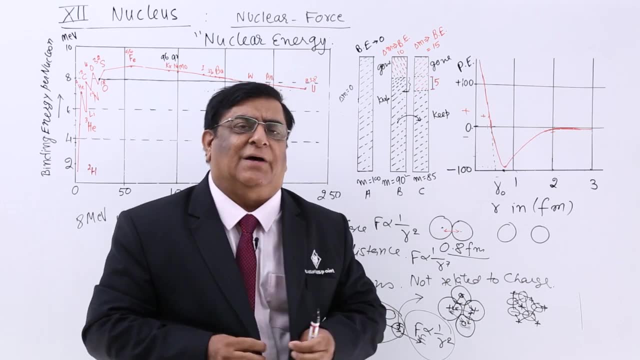 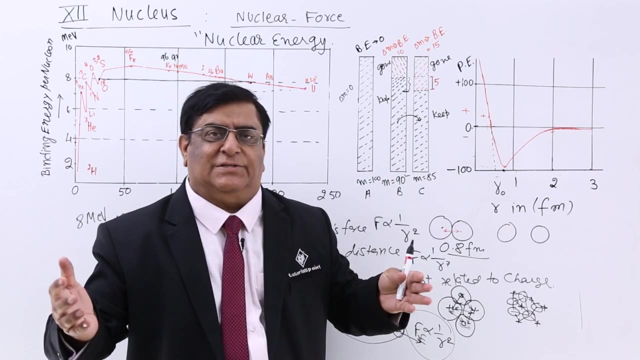 and bring the size smaller. That is why the size is always limited. It cannot go beyond that. It is a very, very natural phenomena and we are seeing this phenomena in our families. When the families grow, there are branches, there are separate houses and larger the size. it is a natural phenomenon. It is a natural phenomena that there will be breakage because of its own weight. It happens in gravitation also. We cannot have an object with a very, very large mass. We have Chandrasekhar limit for that. 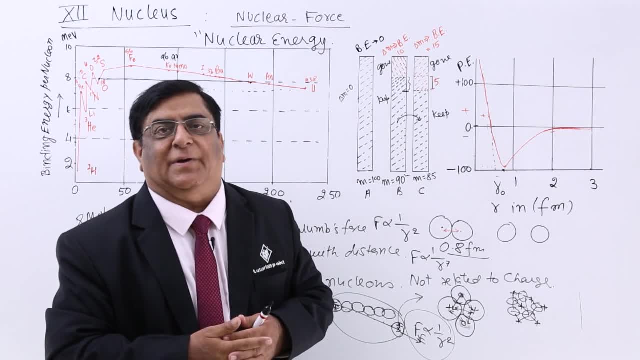 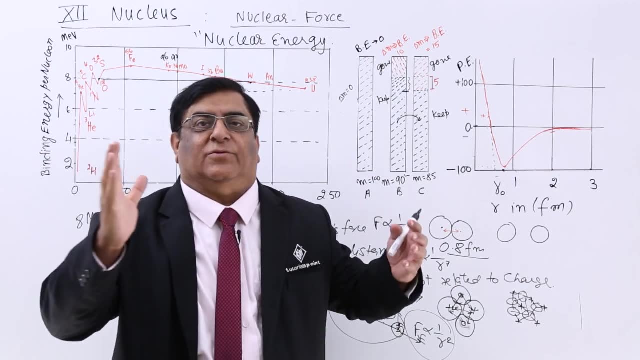 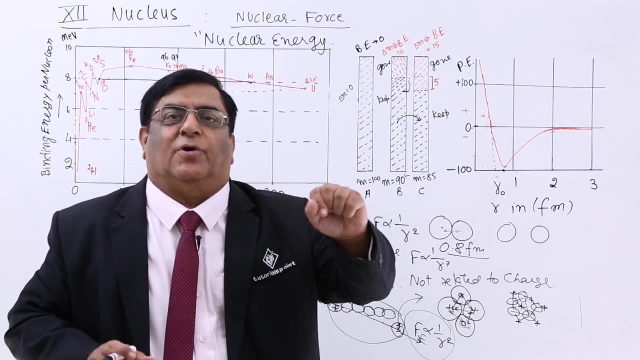 If the mass is beyond that Chandrasekhar limit because of its own gravitational forces in different parts, it separates out, it breaks. Same thing happens here. When size become very large, the force by proton become very high compared to nuclear force. 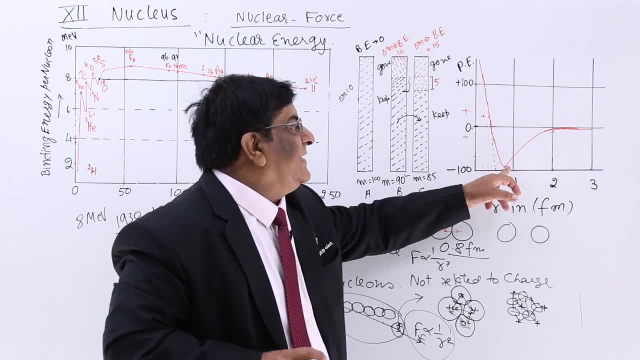 So this is about the nuclear force: a short range, stronger than coulomb, but range is short. Thank you, 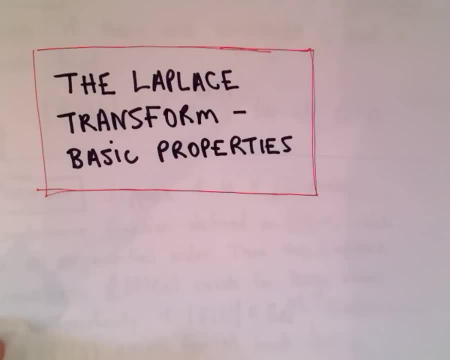 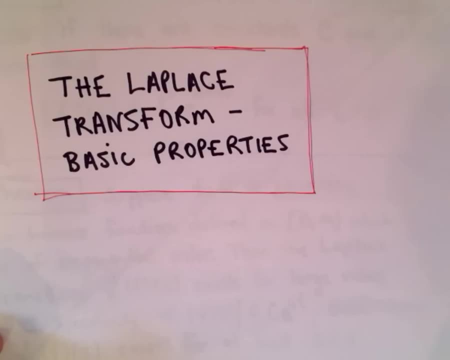 Alright, this video is going to be about the Laplace Transform and some basic properties, So I'm going to give a definition and a couple definitions and a theorem without proof, but then we'll talk about, kind of the one of the big propositions that you use a lot to solve differential equations using the Laplace Transform. 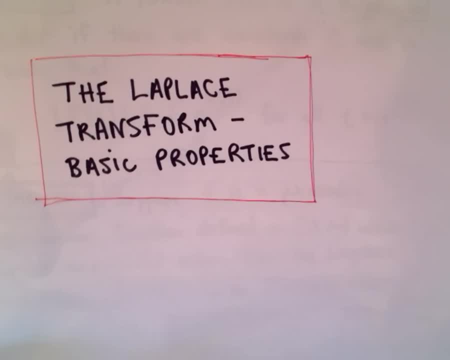 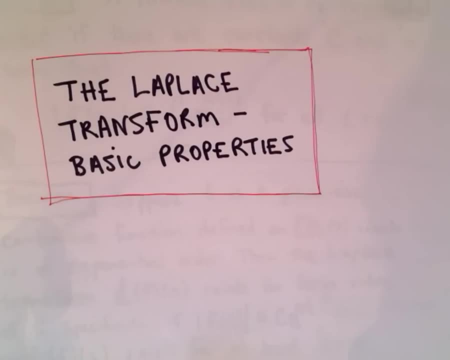 and we will solve that. It's just basically another integration by parts proof. So you know a couple of the theorems in here are important, obviously, Obviously, I don't know that there's anything that mechanical on here, except for the last proposition that's going to be useful.